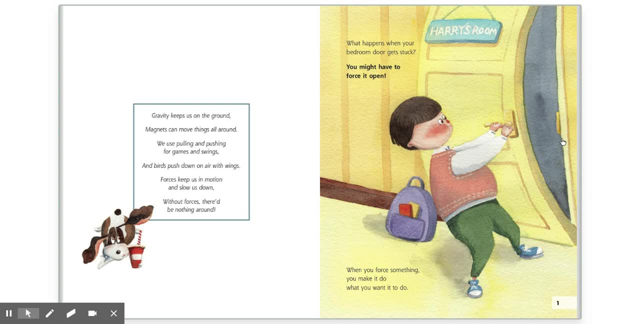 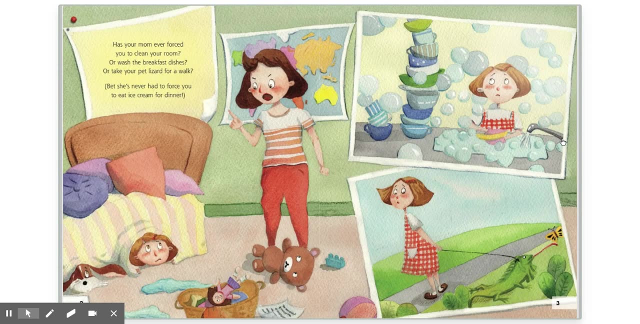 What happens when your bedroom door gets stuck? You might have to force it open. When you force something, you make it do what you want it to do. Has your mom ever forced you to clean your room Or wash the breakfast dishes, Or take your pet lizard for a walk? Bet she's never had to force you to eat ice cream for dinner. 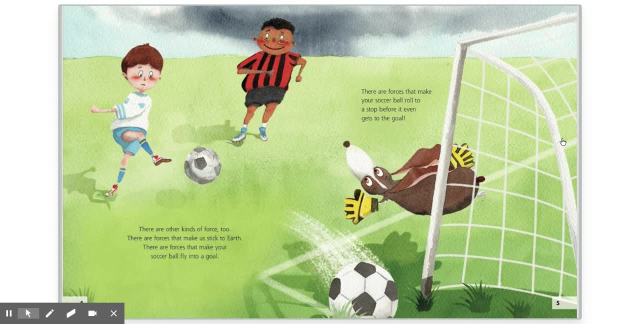 There are other kinds of forces too. There are forces that make us stick to Earth. There are forces that make your soccer ball fly into a goal. There are forces that make your soccer ball roll to a stop before it even hits the ground. 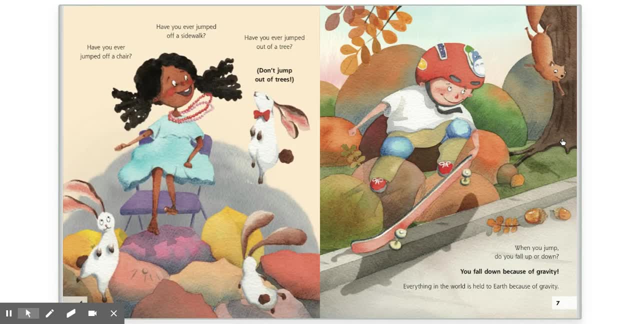 Have you ever jumped off a chair? Have you ever jumped off a sidewalk? Have you ever jumped out of a tree? Don't jump out of trees. When you jump, do you fall up or down? You fall down because of gravity. Everything in the world is held to Earth because of gravity. 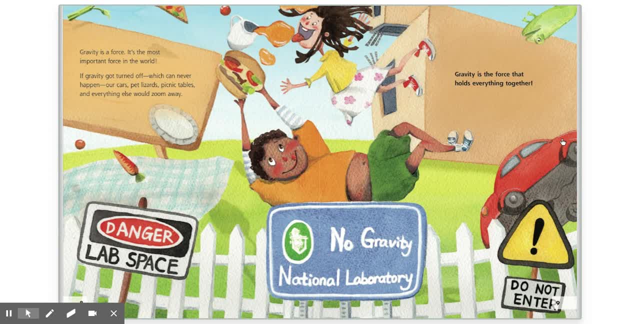 Gravity is a force. It's the most important force in the world. If gravity got turned off, what would happen- Which can never happen? Our cars, pet lizards, picnic tables and everything else would zoom away. Gravity is the force that holds everything together. 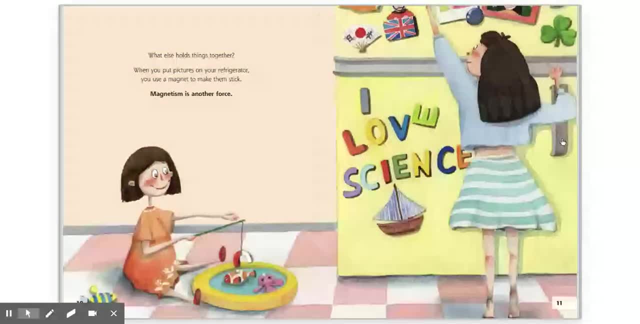 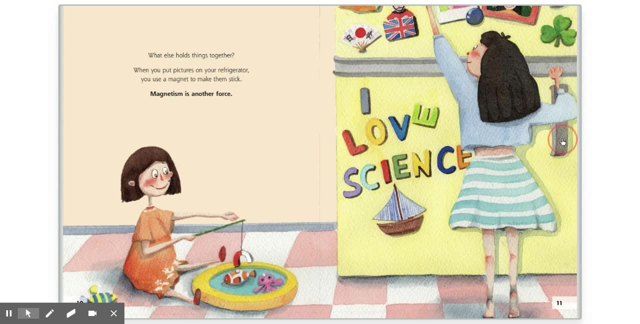 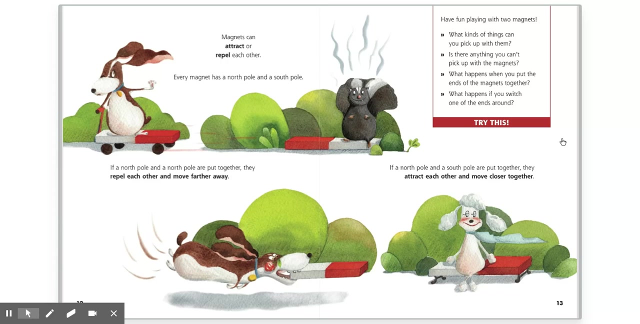 What else holds things together? When you put pictures on your refrigerator, you use a magnet to make them stick. Magnetism is another force. Magnets can attract or repel each other. Every magnet has a north pole and a south pole. If a north pole and a north pole are put together, they repel each other and move further away. 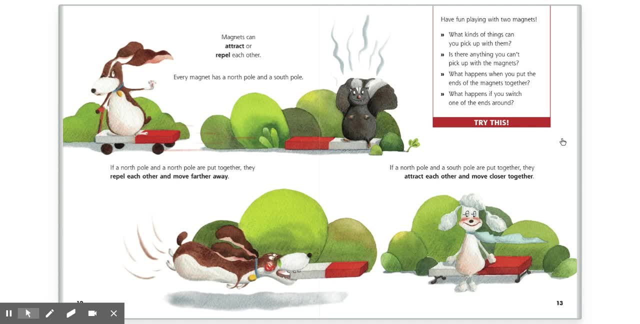 If a north pole and a south pole are put together, they attract each other and move closer. Have fun playing with two magnets. What kinds of things can you pick up with them? Is there anything you can't pick up with the magnets? What happens when you put the ends of the magnets together? 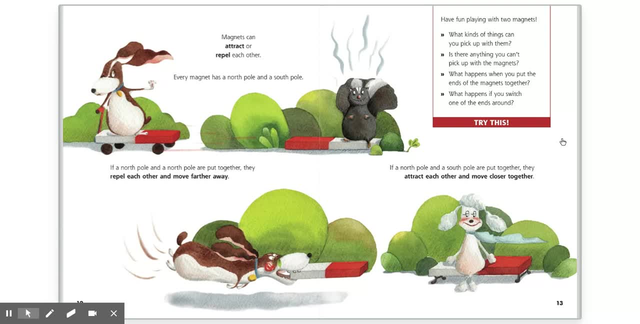 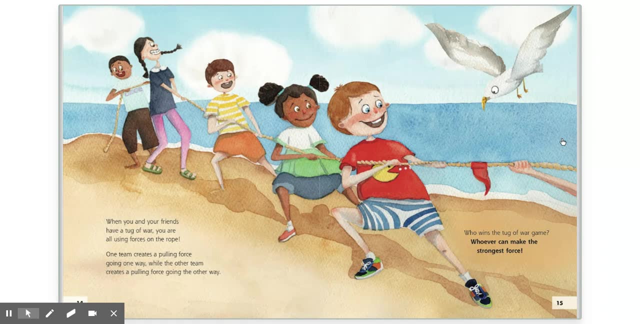 What happens if you switch one of the ends around. Try this: When you and your friends have a tug-of-war, you are all using forces on the rope. One team creates a pulling force going one way, while the other team creates a pulling force going the other way. 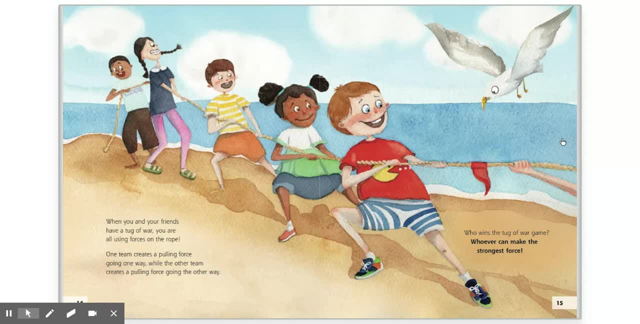 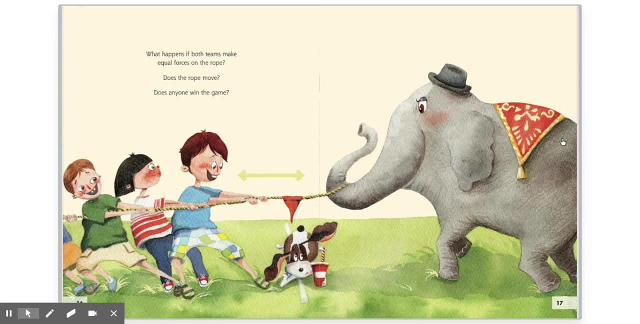 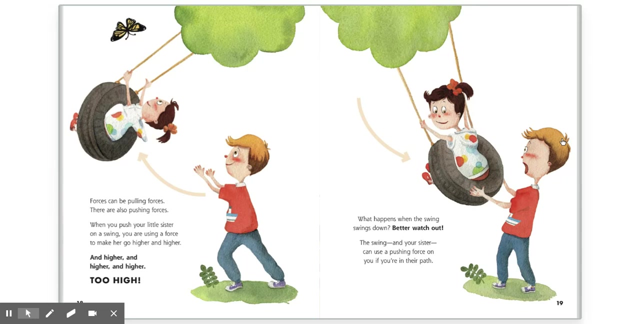 Who wins the tug-of-war game? Whoever can make the strongest force? What happens if both teams make equal force? What happens if both teams make equal forces on the rope? Does the rope move? Does anyone win the game? Forces can be pulling forces. 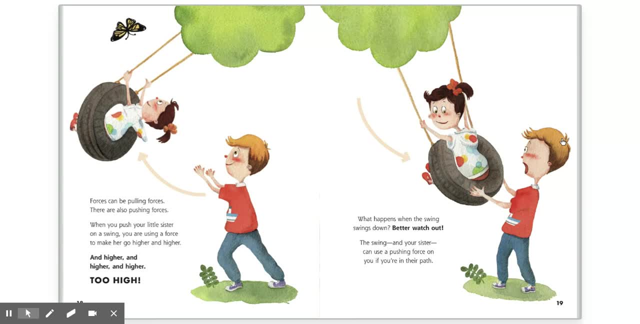 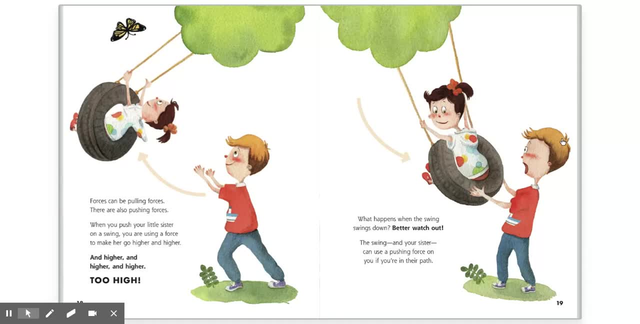 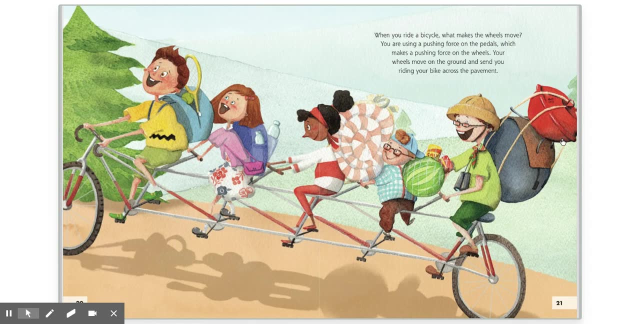 The swing and your sister can use a pushing force on you if you are in their path. When you ride a bicycle, what makes the wheels move? You are using a pushing force on the pedals, which makes a pushing force on the wheels. Your wheels move on the ground and send you riding your bike across the pavement. 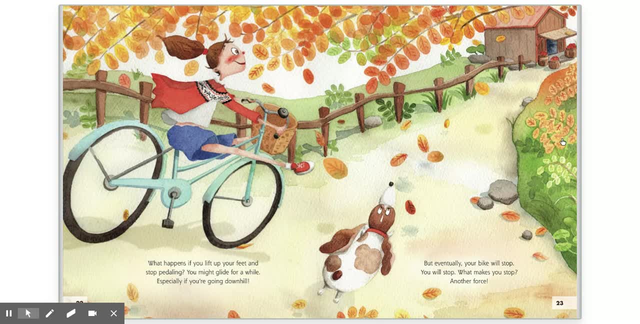 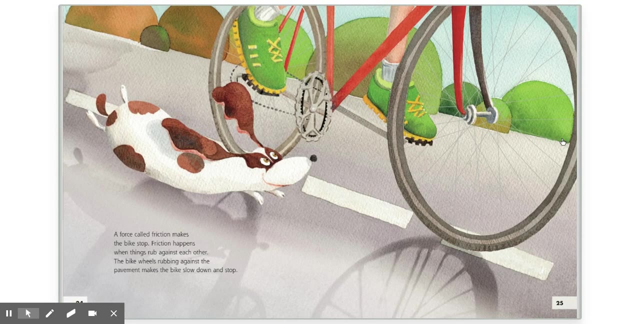 What happens if you lift up your feet and stop pedaling? You might glide for a while, especially if you are going downhill, But eventually your bike will stop. You will stop. What makes you stop? Another force, A force called friction, makes the bike stop. 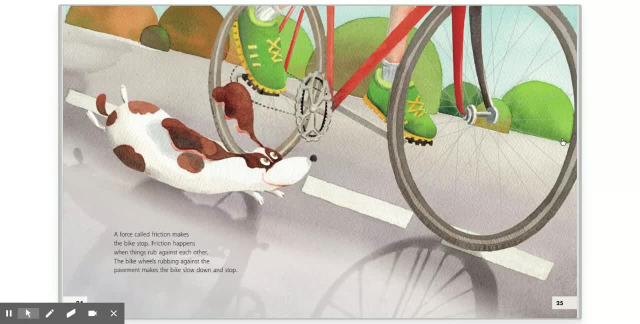 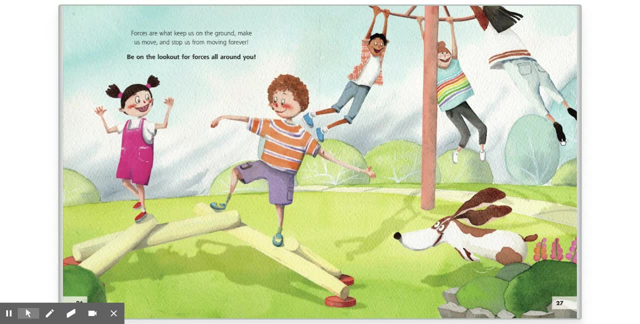 Friction happens when things rub against each other. The bike wheels rubbing against the pavement makes the bike slow down and stop. Forces are what keep us on the ground, make us move And stop us from moving forever. Be on the lookout for forces all around you. 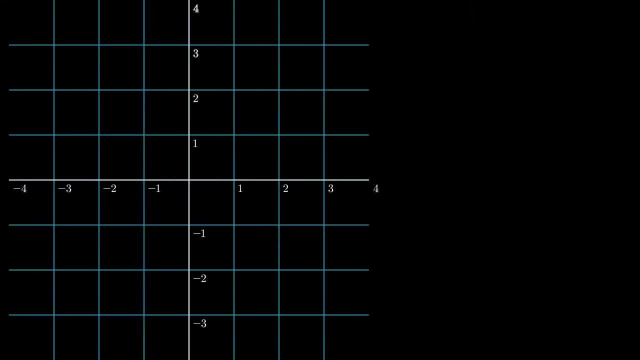 In this first lesson of Calculus 3, we're going to be reviewing vectors in 2D, 3D and the unit vector. This first vector u is going to be 3 in the x direction and 1 in the y direction. 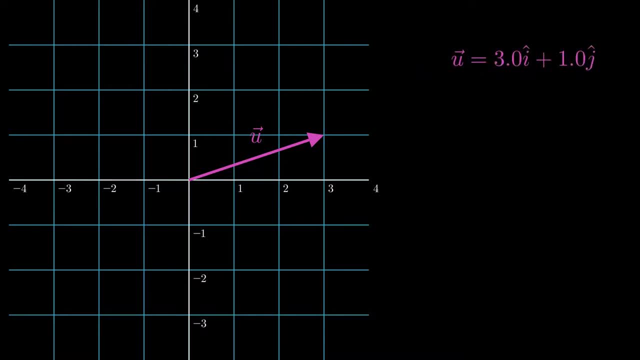 If we move it over to the right here, the component form looks like this: We're going to have a second vector in the third quadrant. There are negative 2 in the x, negative 3 in the y and the component form is going to be negative 2- i-hat plus negative 3- j-hat.